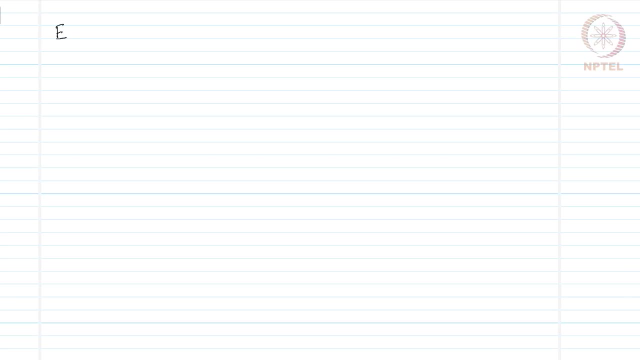 concept of that. Uh, drawing is not that good. let me try to redraw this negative charge distribution. So the negative charge distribution will be symmetric to the nucleus. that means the nucleus will be at the center of it, And when we apply an electric field on this arrangement, 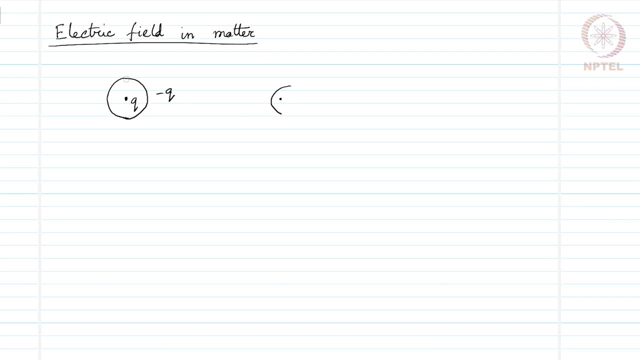 then the system will try to rearrange, rearrange itself in such a way that the electric field is mitigated somewhat. So here we have subjected this to an electric field. this is the positive charge at the center and the negative charge cloud. You can see that the positive charge, that is the 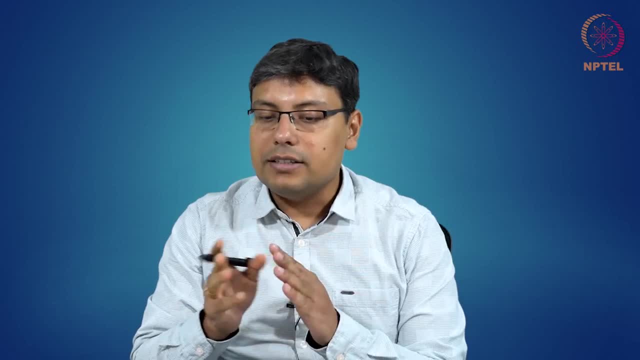 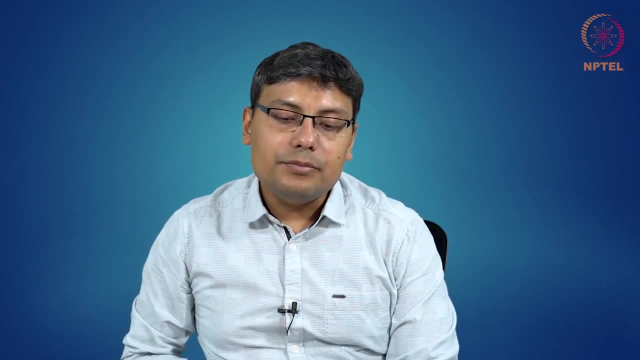 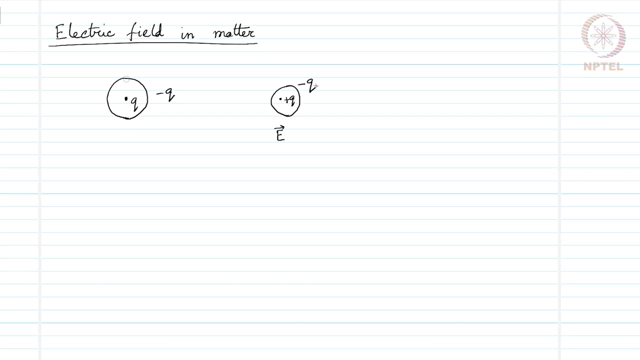 nucleus is no longer at the center of this negative charge cloud. This is the way an atom would respond to an external electric field and similarly you can see some polarization is being developed in a dielectric material. If that happens, then let us try to find out. 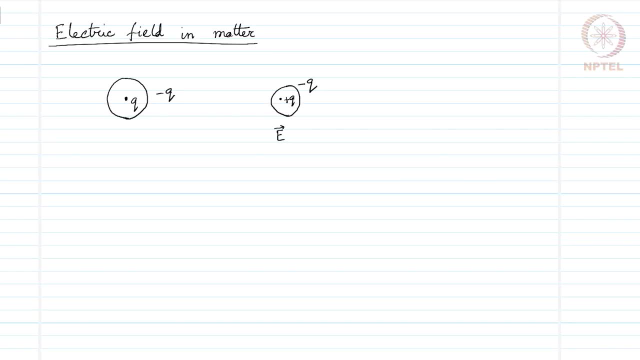 the center of this charge, this negative charge distribution here. Let me get rid of this plus q written from here. let us write, let us write plus q here, And the center of this negative charge distribution will be somewhere here, and the separation between these two is d, So you can see that. 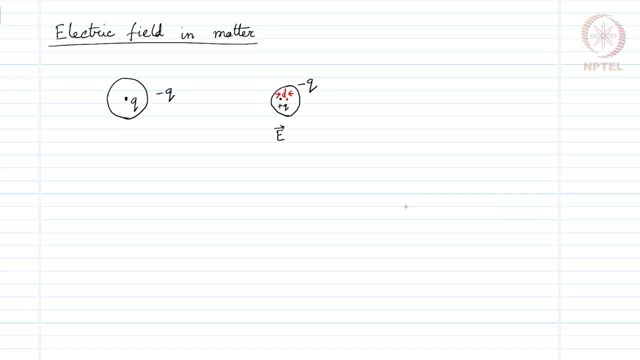 a dipole moment is developed in this atom itself. and let us consider an interesting example. with this idea in mind, We consider a primitive model of an atom consisting of a point nucleus with plus q charge, surrounded by a uniformly charged spherical cloud of electrons, and the radius of that spherical 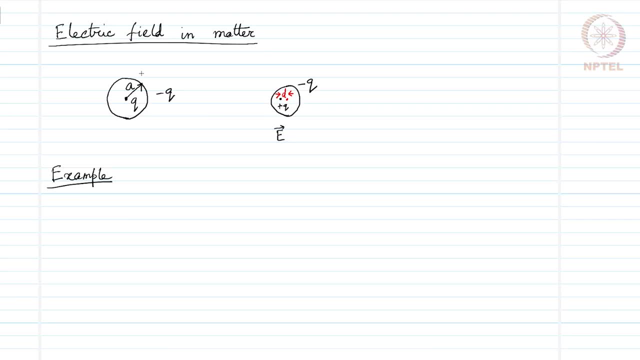 cloud of electrons is a. Now the problem asks us to calculate the atomic polarizability of such an atom. How do we do that? If the equilib if at equilibrium, we consider thatwhen we supply the electric field, this nucleus moves a distance d from. 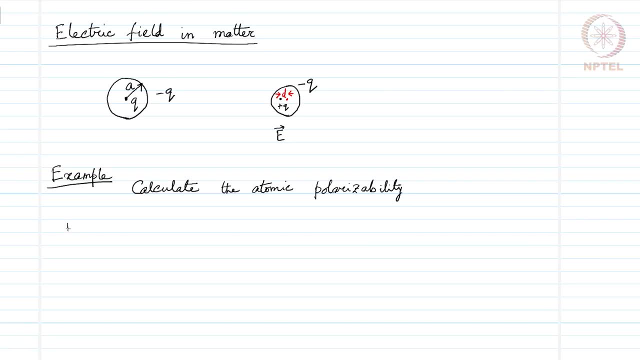 the origin C cliched in the performance, It cores 8 into 6, so we are able to moving the electro fieldav him to a distance more k k k, that would be their distance. 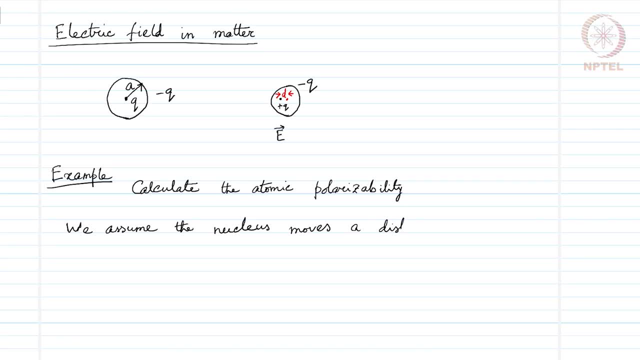 So you have this point: Dお succeed in the supposeفي 1, ok, purchased to. So if that happens, then the electric field due to this dipole, the magnitude of that is 1 over 4 pi. epsilon naught q, d over a cubed, where d is the distance between the positive. 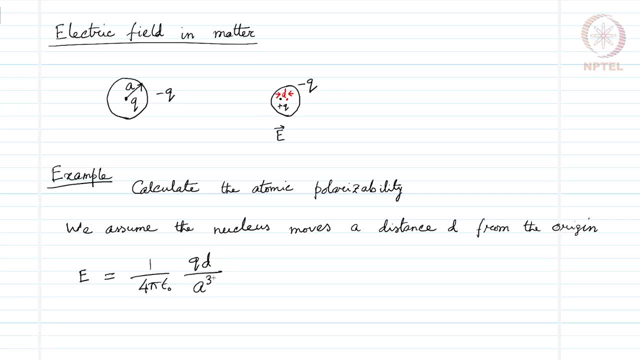 charge and the negative charge center, and a is the distance, a is the radius of this spherical electron distribution. And so this is the electric field due to the dipole. So we can write in terms of dipole moment. this quantity is nothing, but well, let us write down the dipole moment corresponding. 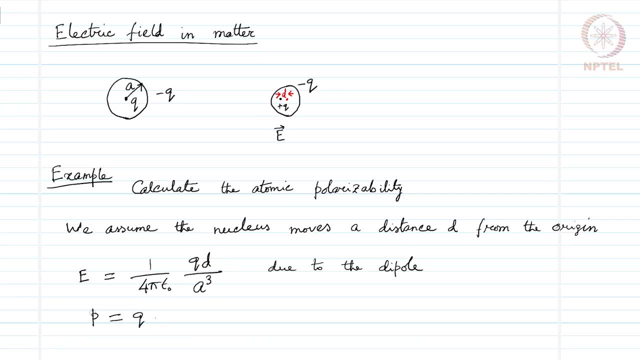 to this, the magnitude of the dipole moment can be written as: p equals q times d. And if we now express this dipole moment in terms of this electric field, we can write it as 4 pi. epsilon naught a cubed times. 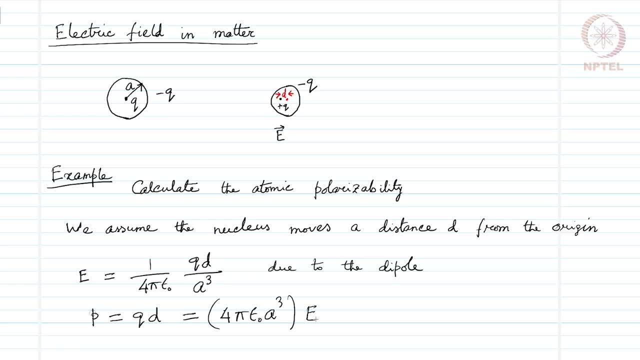 The electric field that we have, So the atomic polarizability we are supposed to calculate. If we express atomic polarizability as alpha, That would be equal to 4 pi. So pi epsilon naught a cubed. that is 3 times epsilon, naught times the volume of that atom. 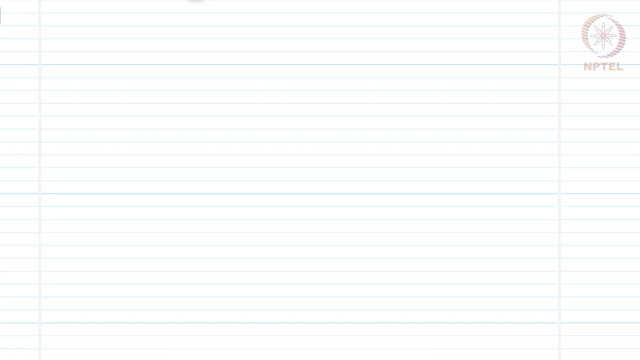 And if we consider a completely asymmetric molecule, Then we can write the dipolethis, atomic polarizability, as a tensor which obeys thismatrix equation P, x, P, y, P, z. this column vector equals: alpha x, x, alpha x y, alpha x z, alpha y, x, alpha y. 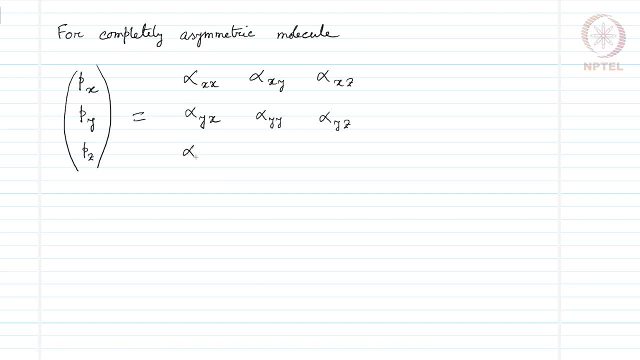 y, alpha y z, alpha z, x, alpha z, y, alpha z, z, Multiplied with the electric field column vector E x, E, y and E z. thishappens when we have an asymmetric molecule at hand, So the atomic polarizability is no longer a scalar. 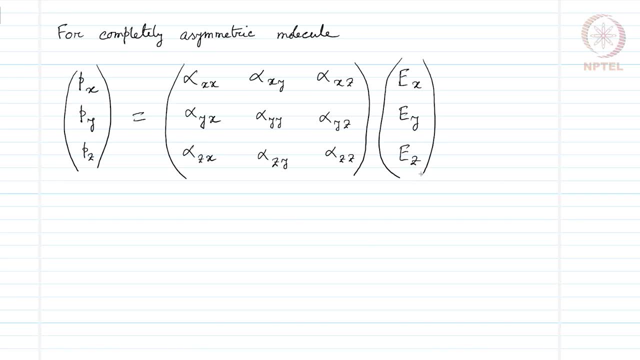 it is rather a tensor, and thismatrix equation holds good relating the atomic dipole moment and the electric field. Now let us consider the alignment of a polar molecule under the influence of external electric field. 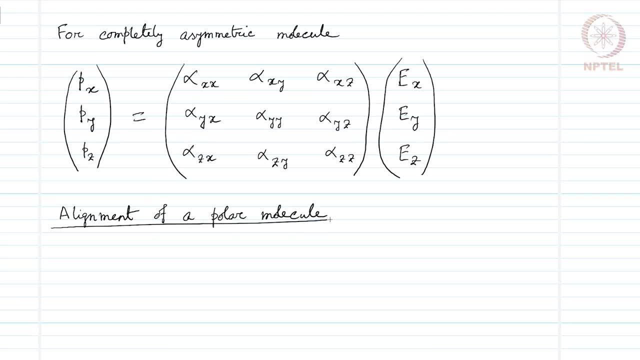 consider water molecule for simplicity. We all know about water molecule. How does a water molecule look? There is a big oxygen atom- this is our oxygen atom- and there are two hydrogen atoms- The hydrogen atoms we are going to colour as blue. let us consider: 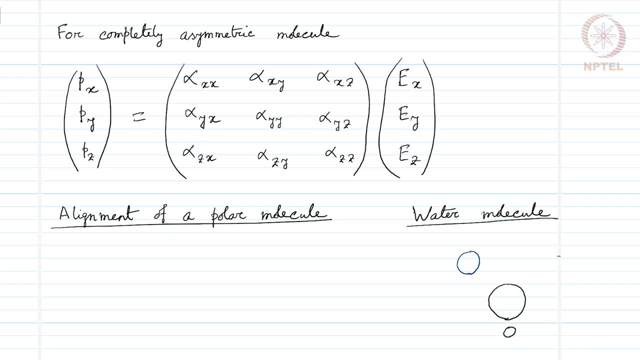 this to be one hydrogen atom and this to be another hydrogen atom. And if I connect the nucleus from the hydrogen atom to oxygen atom, atom to oxygen atom, we get an angle. here this angle is 105 degree. So let us mark the atoms. 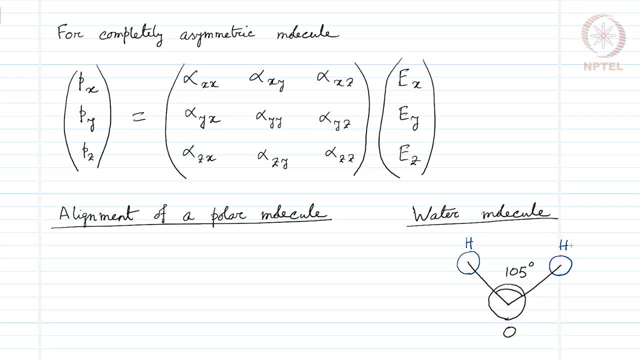 this is a hydrogen atom. this is a hydrogen atom and if we have this kind of an arrangement, we can clearly see that. So oxygen is 2 minus and hydrogen is. these are positively charged, So this makes an ionic compound, but a polar compound. So we can clearly see that due. 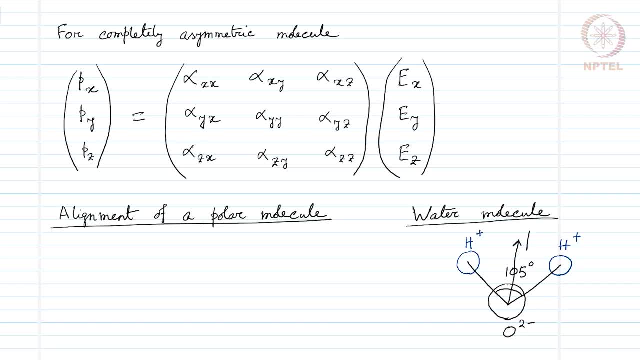 to this. the dipole moment will point along this direction. that would be the direction of the dipole moment vector. Let us consider this kind of a situation a bit simplified one. Let us consider a conventional dipole with plus, q and minus q charges. Here we have plus q charge, here we have minus. 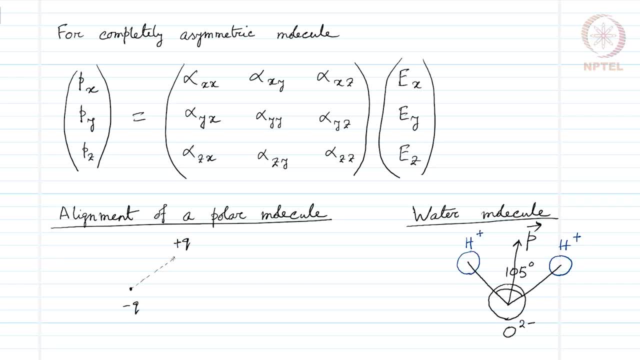 q charge and if that makes a molecule an ionic compound. So this is the origin of the coordinate system O and the separation is the vector D. now we consider applying an electric field along this direction. If we consider that, then what is going to happen? this electric field is going to apply a force on this atom. 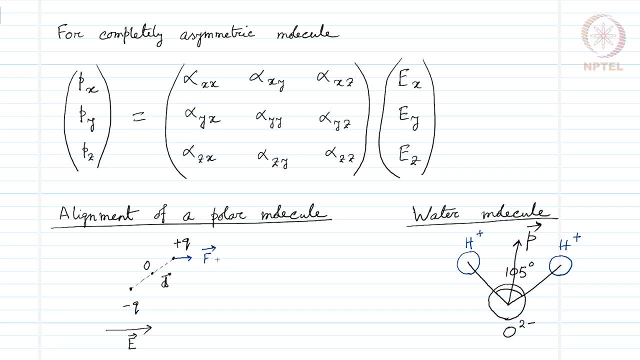 in this direction. So, in that case thing, we accept the hard connection from the positive point and we consider: which can be Devin's, Let us call it F- plus same amount of force on this atom. in this direction, let us call. 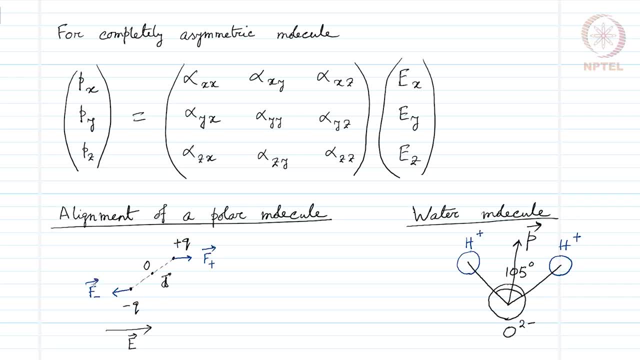 it F minus, and under the influence of these two forces it is going to develop a torque for the geometry given here. If we call that torque as n, that would be given as r plus vector, cross, F plus vector plus, r minus vector, cross, F minus vector and that turns out to: 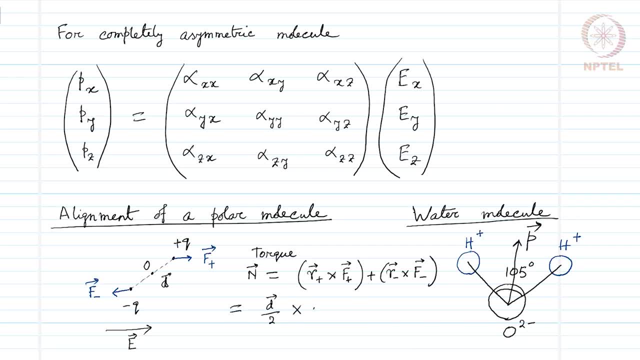 be d over 2.. Cross Q e plus minus d over 2. cross minus Q e, which is essentially Q d. cross the electric field. In other words the torque n is given as the dipole moment cross product with the applied electric field. This is the amount of torque this molecule, due to this arrangement of its 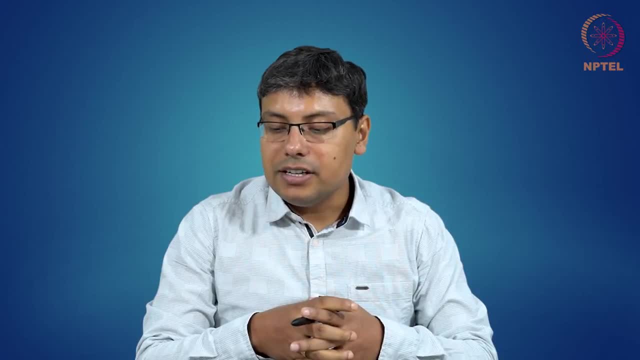 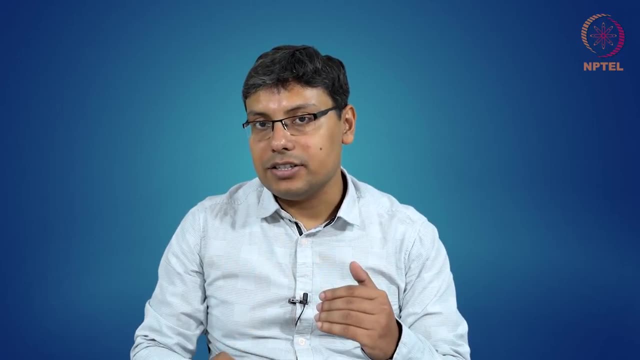 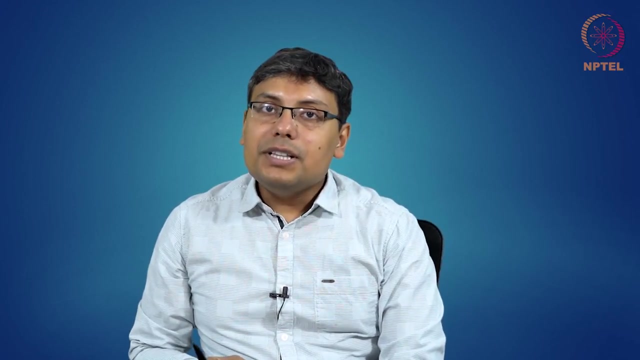 subject to compared to the direction of the electric field, will experience and, if possible, if this torque is enough to align it along the direction of the electric field, it will get aligned along the direction of the electric field. So for a simple atom, we have considered that the simple atom can develop a dipole moment. 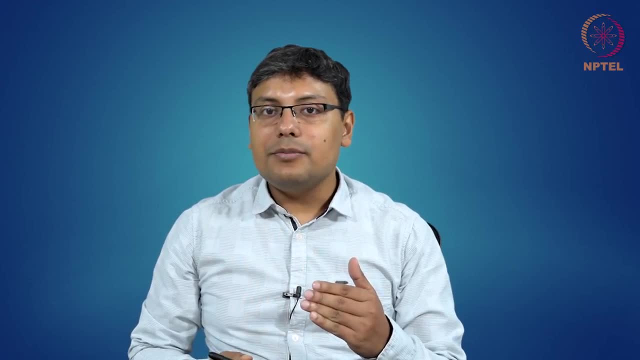 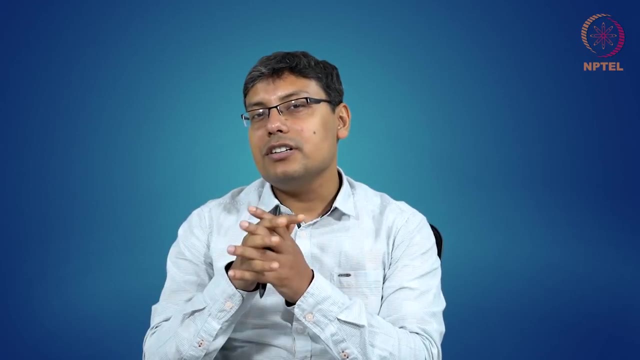 develop a polarization subject to an electric field, by shifting its positive charge center and the negative charge center. that means the electron cloud will move somewhat and it will develop a polarization. In case of polar molecules, its even more interest thus that they need to be polarized to possible. gy probe memories. 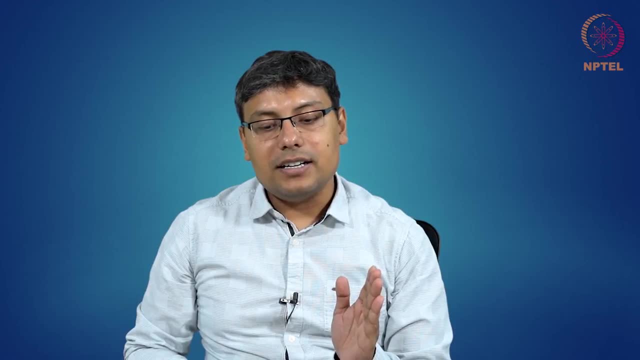 So the set at two polesτhe polarization is going to happen for two donen reaching be positive charge center. So that means, in this case, hilarious electric field that is leaving this particular. We can see that it can align itself along the direction of the electric field, So it 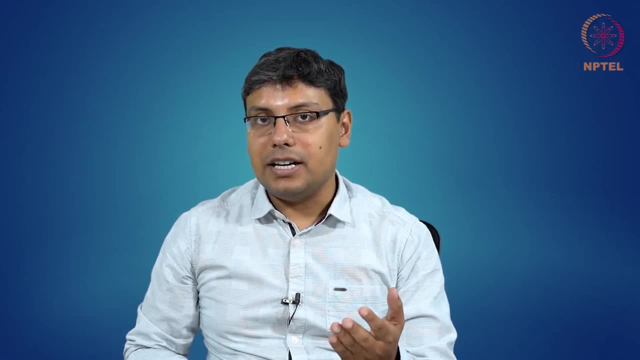 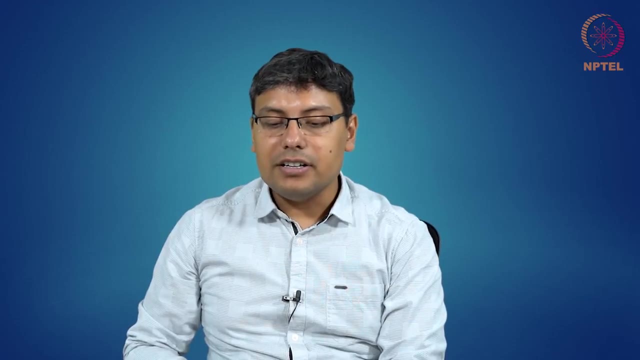 can rotate that molecule, if that is allowed, ifthat polarmaterial, the polar molecule, forms a liquid, not a solid. in case of a solid, tilting itself is very difficult, although not impossible. So in case of a liquid it is very easy to align that molecule in the direction of the 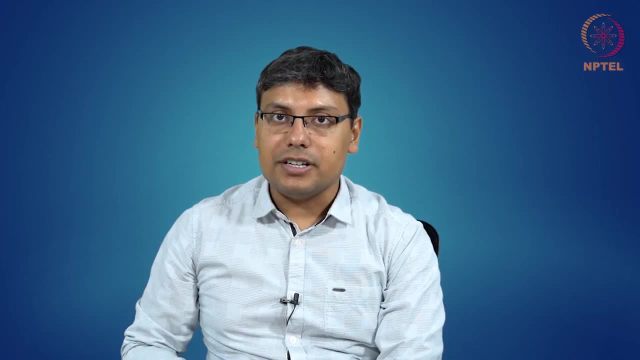 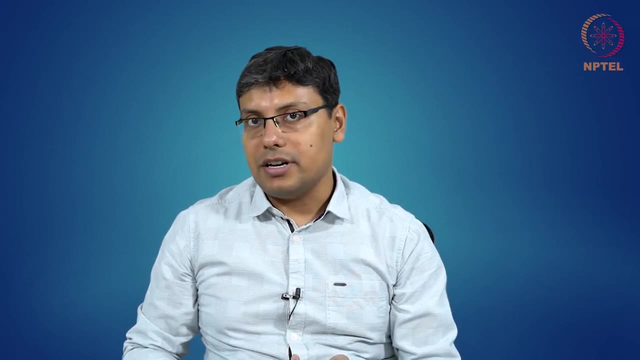 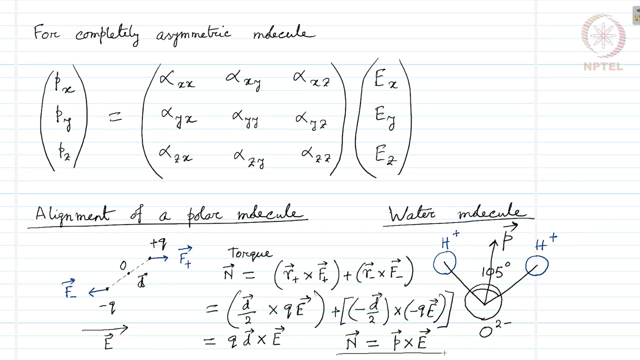 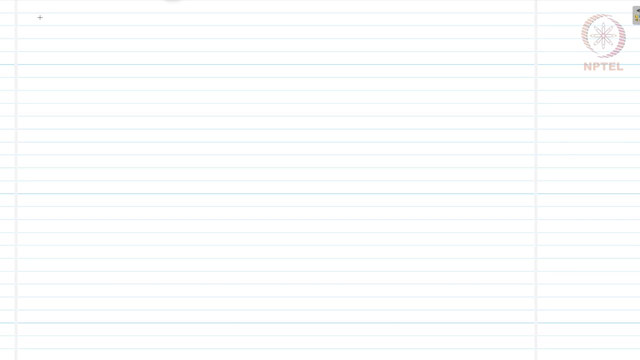 electric field and that develops a polarization in that material. So we have made some effort to microscopically understand how a material can be polarized. Now, in this consideration for this moleculethe polar molecule that aligns itself if we consider that the electric field is non uniform. 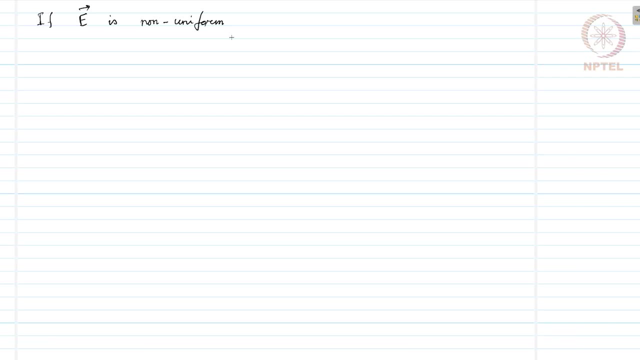 So this: we will not have F plus and F minus exactly balancing each other, So the magnitude of F plus will not be equal to the magnitude of F minus. in that case we will have a total force on this molecule And that will be obviously the difference between these two forces. we 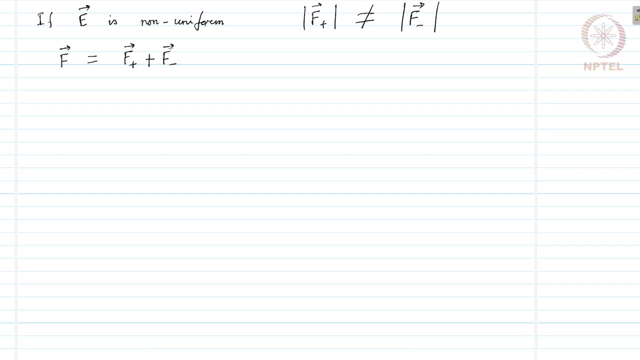 are summing the forces because they are opposite in sign, and so the total force is given by this, which is nothing but q times E plus minus E minus. So E plus is the electric field on the positive charge and E positive ion and E minus is the electric field on the negative ion, and that 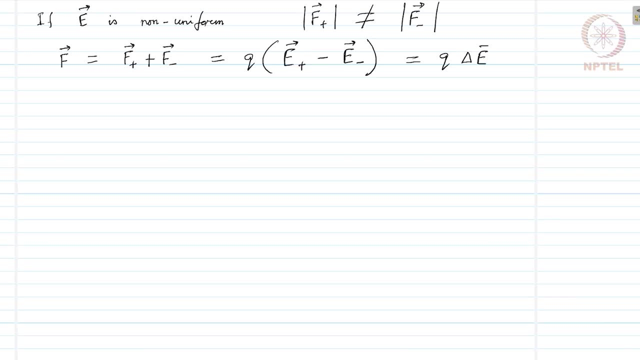 is q delta E. delta E is just E plus minus E minus. So let us consider the x component of this delta E. delta E x equals gradient of E, x, dot the distance vector d and assuming the electric field on the positive charge. So this is the electric field on the negative. 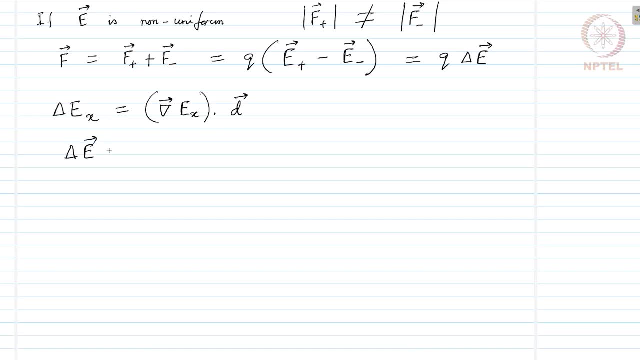 field in x direction. So delta E can be given as d dot del applied on the electric field vector. That means the total force on this molecule that is given as the dipole moment dot del vector times the electric field. ok, After having discussed this, let us consider polarization. Polarization is represented: 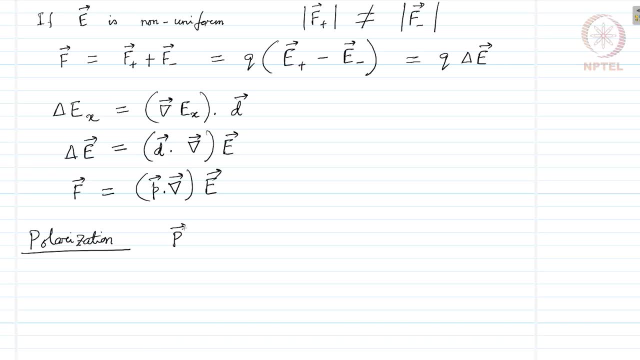 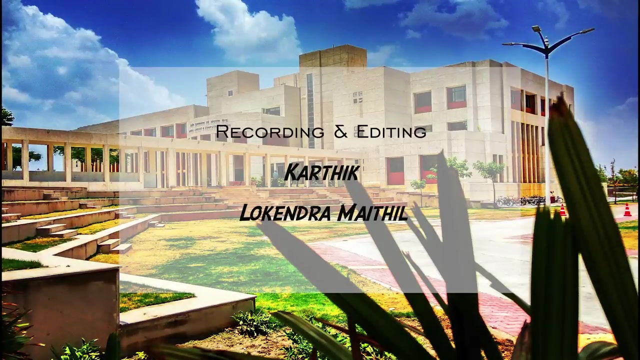 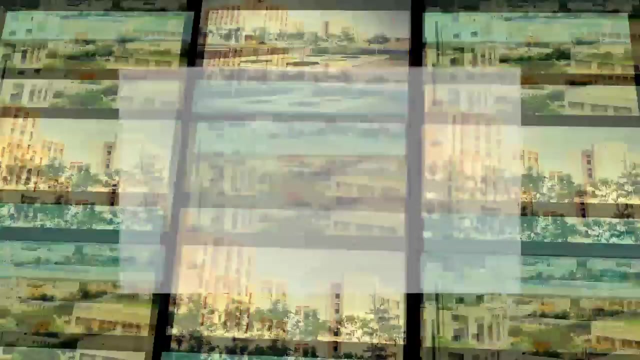 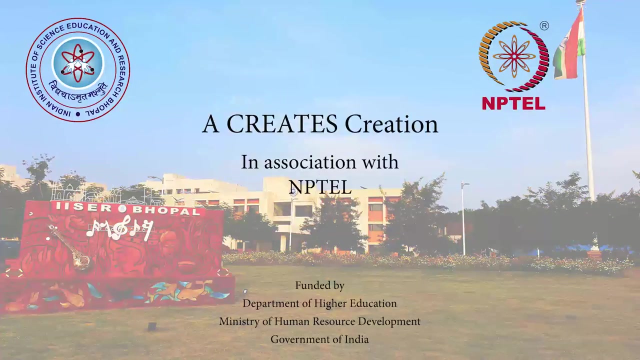 by capital P vector and small p vector is the dipole moment vector. So this is the dipole moment vector and where p is the dipole moment vector. So let us consider this and unit volume in a material. Thank you for watching.